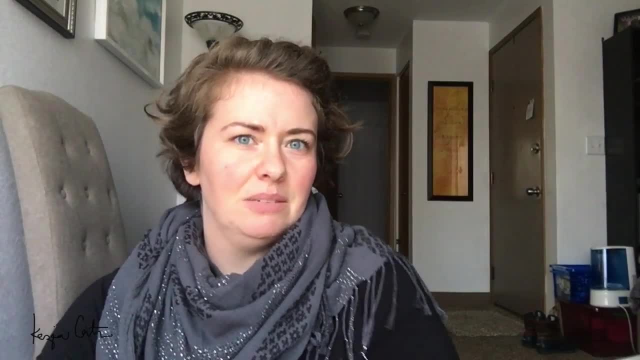 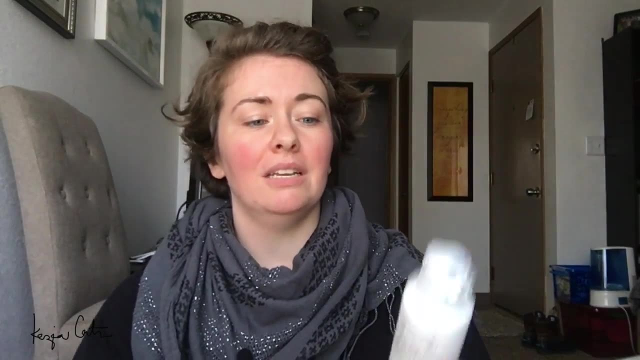 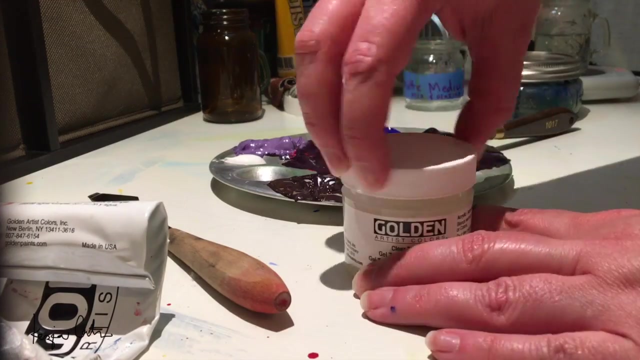 But then again I like to mix my own colors, usually unless I'm looking for, like, an iridescent type color. I don't have a preference between fluids or heavy bodies, but I do tend to water down, or even if I don't use water, water down the paint with something else, so that- because it's not just- 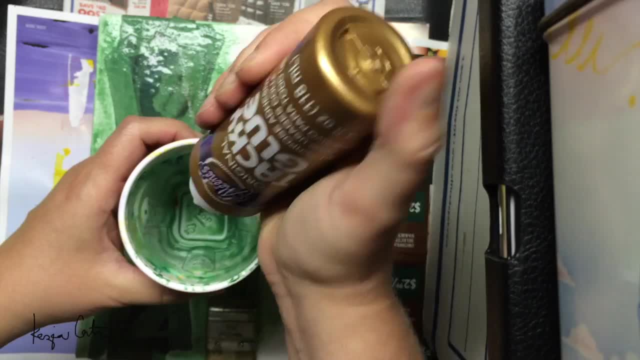 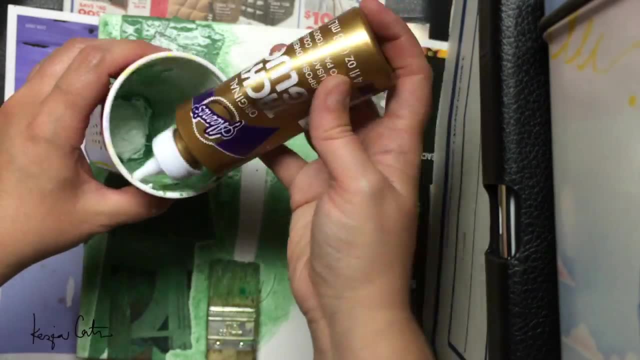 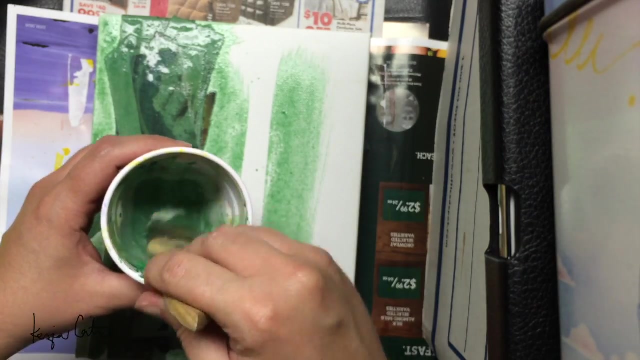 I can't just paint with the paint straight up. you know what I mean. Fluids are good for topical like glazing layers or, if you like to do, billions and billions of really thin layers that build up on each other. But you can mix it with a medium like a gel medium or a gesso to thin it. 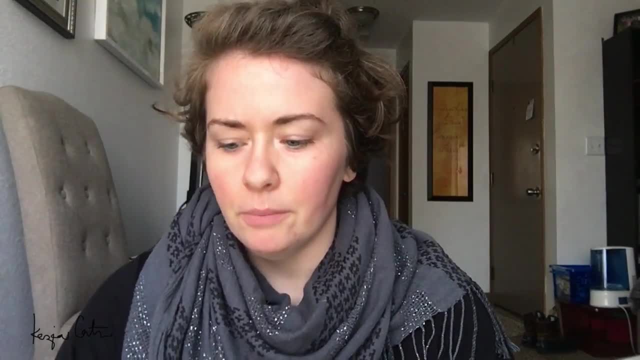 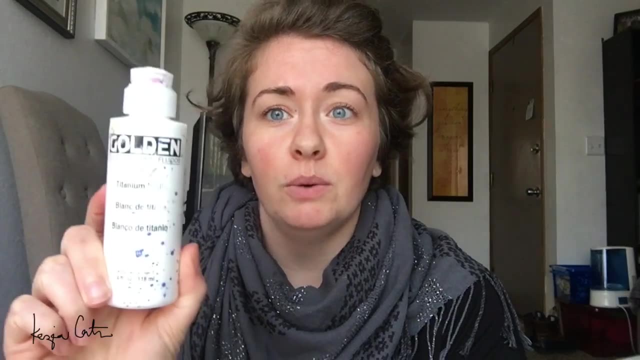 out, You don't have to add water. Speaking of adding water, though, if you like to add lots of water to your paint to make it super thin, you might as well go with a fluid then, because you won't have to add as much water, because the more water you add, the more water you're going to get. 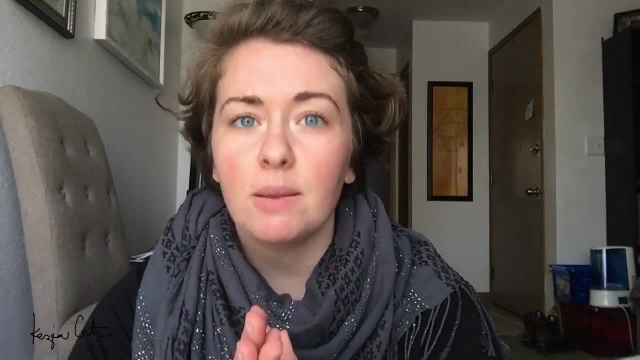 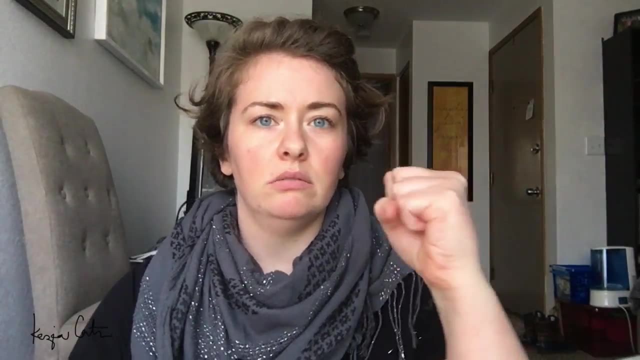 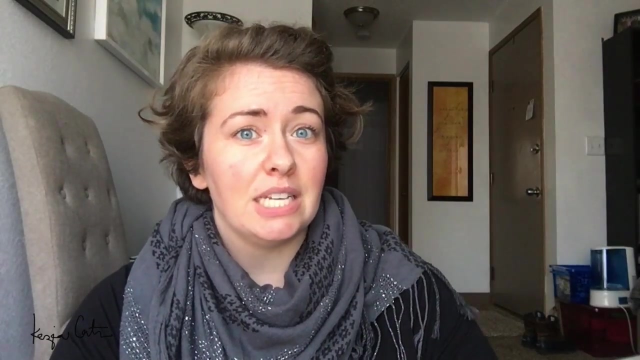 The more water you add to a paint, the less your pigment is going to stick to your surface. The general ratio would be like a one-to-one, like if you had had this much paint, you add the same amount of water. However, there are of there are ways to get around that, where you can seal your. 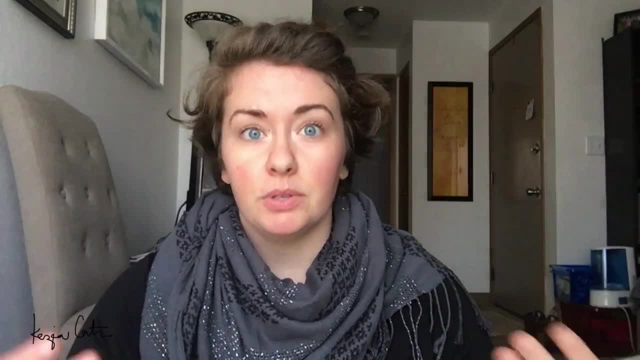 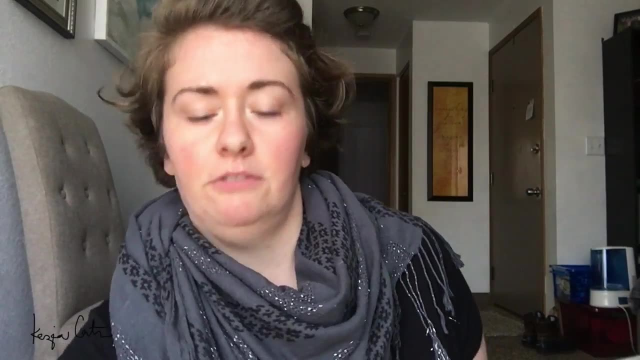 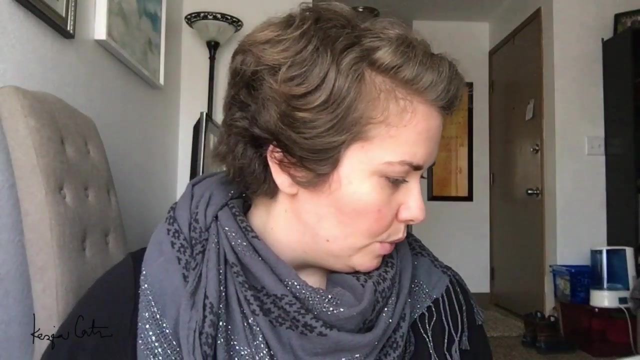 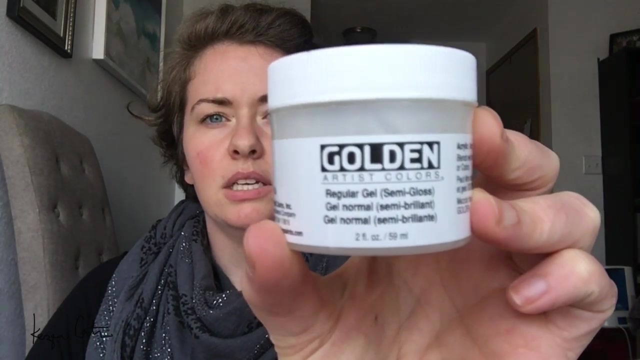 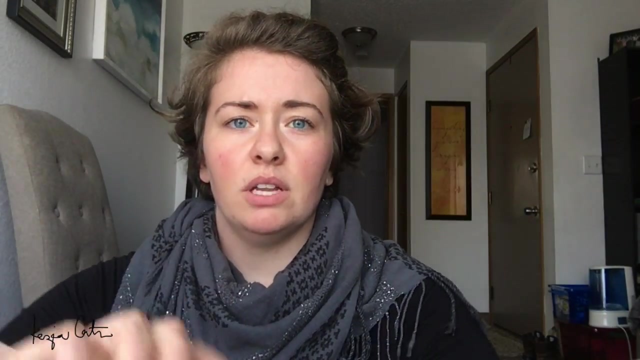 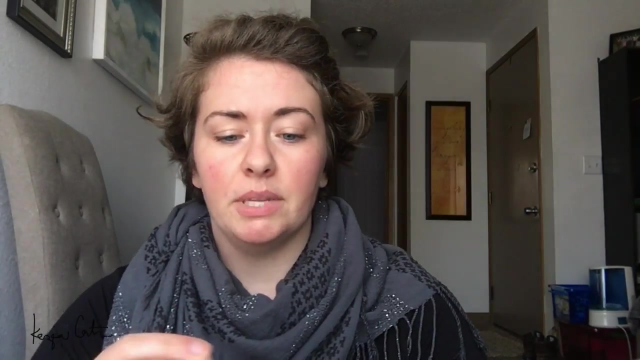 painting with like an acrylic finish or something to help strengthen the binding quality. Now, I think the most versatile of the two are is the fluid. The fluid is the most versatile of the two. I think the most versatile of the two is the fluid because even though it's thinner, you can always mix it with. I found it okay. this is a. this is a acrylic gel medium. this is like- let me see, can you read it? gel, semi-gloss. This is an example of a medium that you can mix with fluids that, I mean, this is almost. I mean, it's just white stuff. Most of them are tinted white, but some of them you can get that are